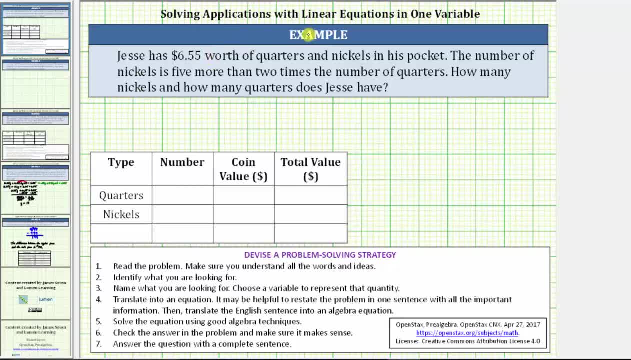 In this video we will solve an application problem using a linear equation and one variable. We will also reference the problem solving strategy outlined here below, where step one is to read the problem: Jesse has $6.55 worth of quarters and nickels in his pocket. 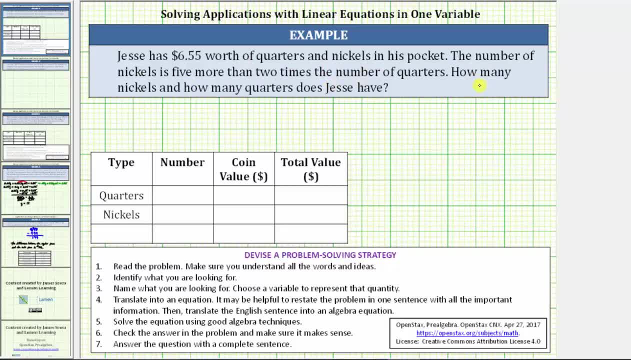 The number of nickels is five, more than two times the number of quarters. How many nickels and how many quarters does Jesse have? The next step is to identify what we are looking for and then, step three: name what we are looking for and choose a variable to represent that quantity. 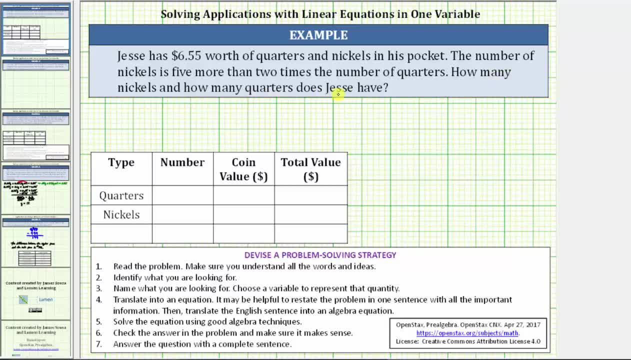 We are looking for the number of nickels and the number of quarters that Jesse has, And because the number of nickels is five more than two times the number of quarters, let's use a variable q for the number of quarters, Because the number of nickels is five more than two times. 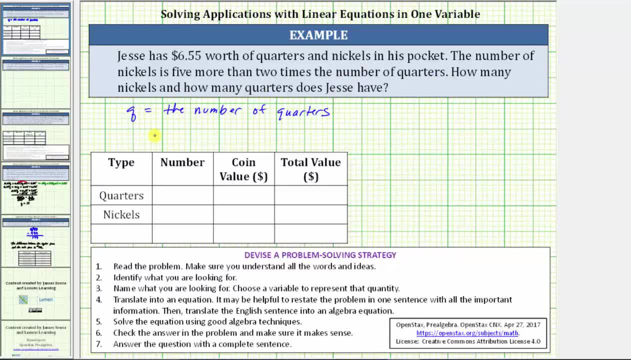 the number of quarters and q is the number of quarters, we can use the expression two q plus five to represent the number of nickels. Again, if q is the number of quarters, two q plus five does represent five, more than two times. 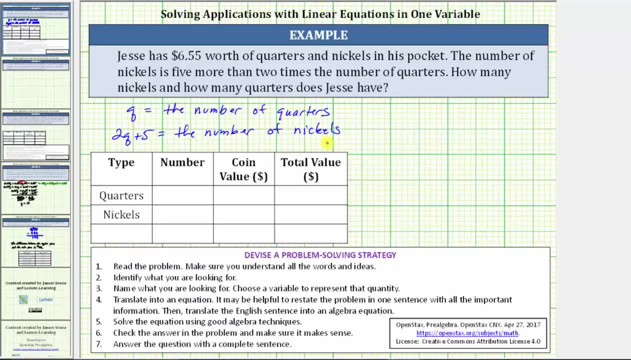 the number of quarters From here, because we know the total value of all of the coins is $6.55,, we will use this table to help us determine an expression for the total value of nickels, of the number of quarters and for the total value of the number of nickels. 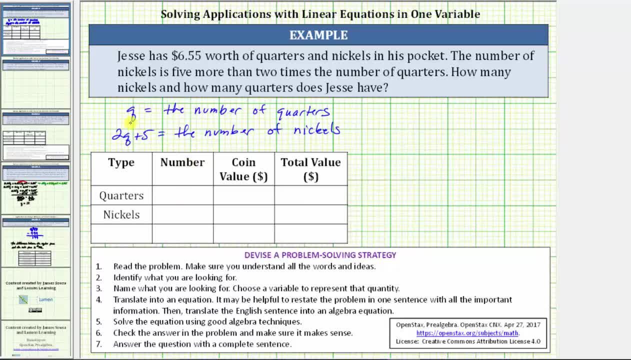 So, looking at the row for quarters, the number of quarters is represented by the variable Q. The coin value of a quarter in dollars is $0.25,, which means the total value of all the quarters is $0.25 times Q or just 0.25Q. 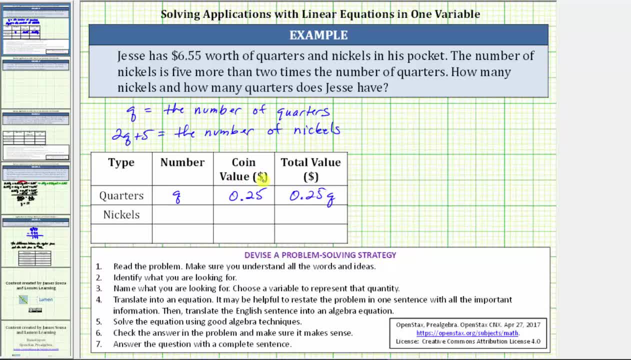 Now I do want to mention: if the coin value was in cents rather than dollars, the coin value for a quarter would be 25 cents and therefore the total value in cents would be 25Q, not 0.25Q. And now for nickels. 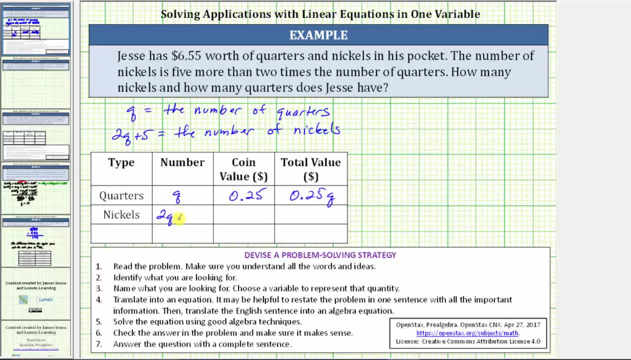 the number of nickels is represented by the expression 2Q plus five. The value of a nickel in dollars is 0.05, which means the total value of all the nickels is 0.05 times the quantity 2Q plus five. 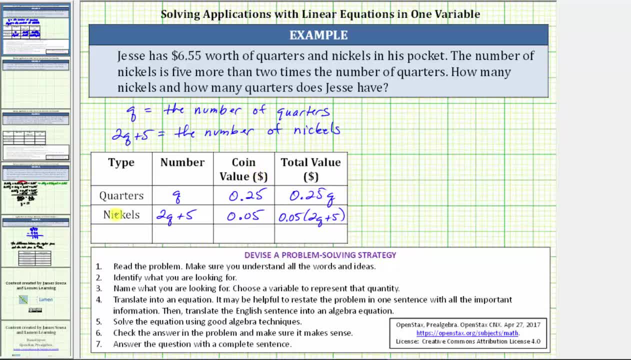 Again, if we were to use cents rather than dollars, the value of a nickel would be five cents and the total value of all the nickels would be five times the quantity 2Q plus five, which again would avoid decimals. The total value of all the coins is $6.55,. 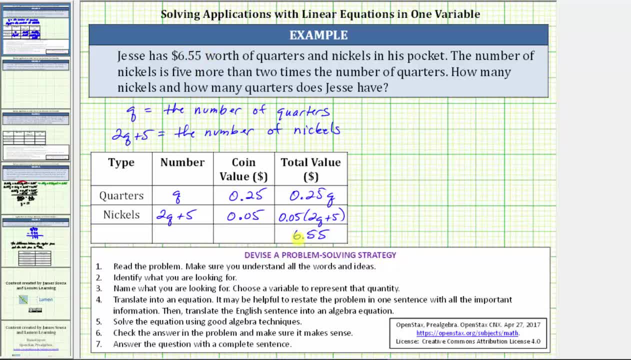 which we will record here. If we were using cents, $6.55, would be $6.55.. And now for step four. we want to write an equation which we can do from this last column here: The value of the quarters plus the value of the nickels. 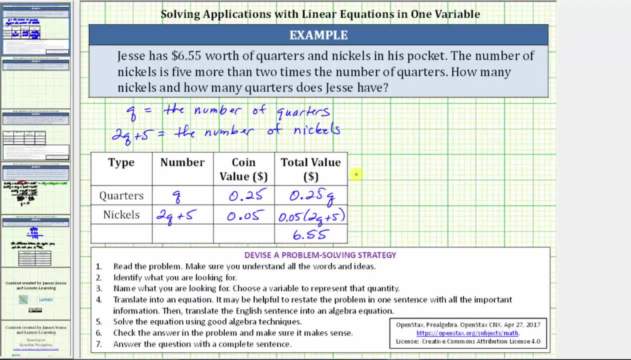 must be $6.55.. This gives us the equation 0.25Q plus 0.05 times the quantity 2Q plus five must equal 6.55.. Let's solve this equation on the next slide, And again I do want to mention 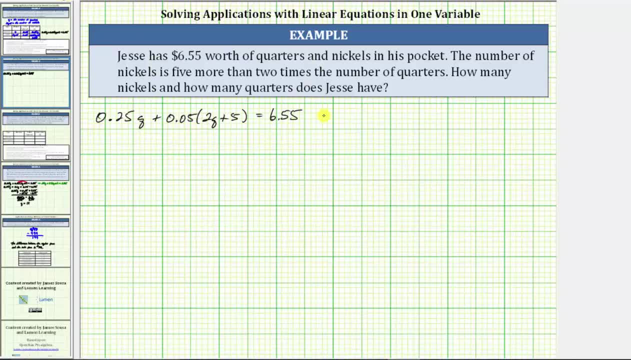 if you were to use cents rather than dollars, the equivalent equation would be: 25Q plus five times the quantity 2Q plus five equals 655.. But our text uses the equation with decimals, so we'll go ahead and solve this equation here. 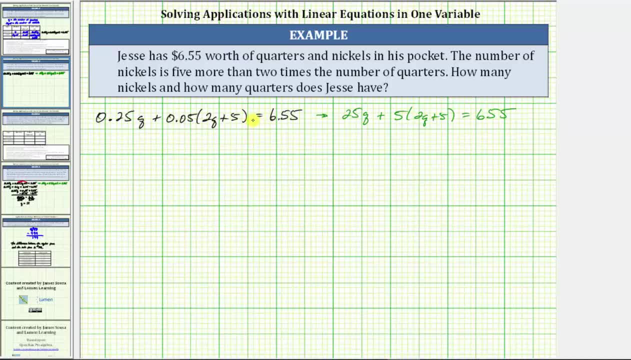 The next step is to simplify both sides of the equation. we simplify the left side by clearing the parentheses and combining like terms, which means now we distribute 0.05.. This gives us 0.25Q plus 0.05 times 2Q is 0.1Q. 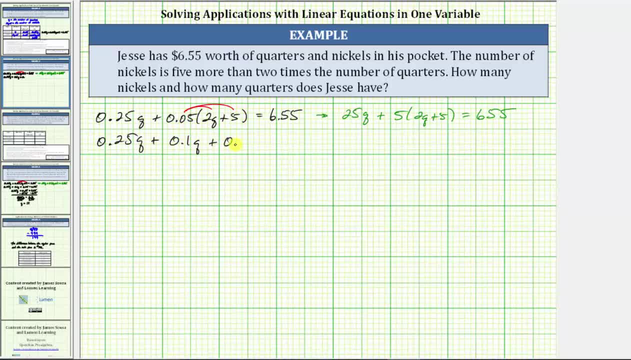 plus 0.05 times five is 0.25.. Combining like terms on the left, 0.25Q plus 0.1Q, is 0.35Q. From here we could clear the decimals from the equation by multiplying both sides by 100. 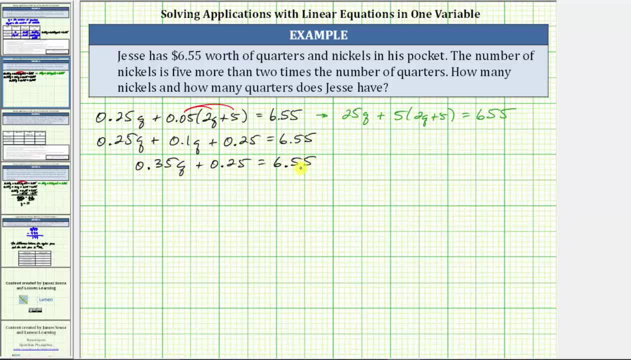 Let's go ahead and solve the equation with the decimals. The next step is to add or subtract. to isolate the variable term on one side of the equation, To isolate 0.35Q, we need to undo this addition by subtracting 0.25 on both sides of the equation. 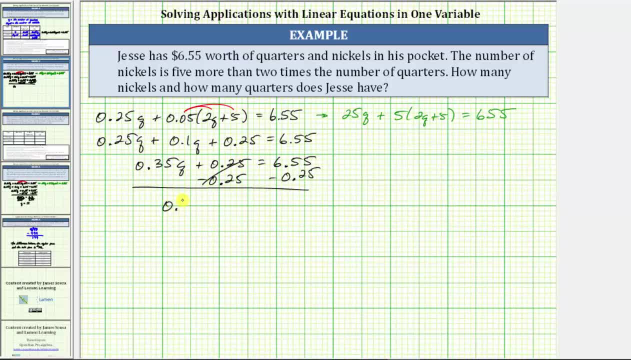 Simplifying this difference is zero. We have 0.35Q. equals on the right. 6.55 minus 0.25 is 6.3.. The last step is to multiply or divide, to isolate Q and solve the equation for Q. 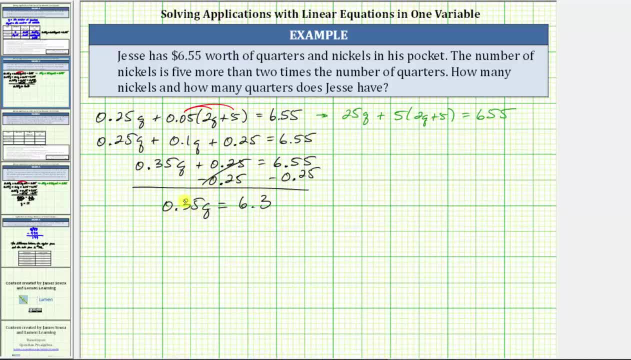 0.35Q means 0.35Q. 0.35Q means 0.35Q, 0.35 times Q. To undo the multiplication and solve for Q, we divide both sides by 0.35.. On the left, this quotient is one. 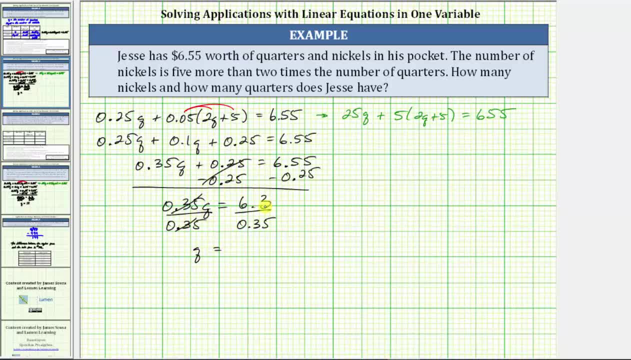 One times Q is Q On the right. 6.3 divided by 0.35 is equal to 18.. So now we know the number of quarters is 18.. Before we determine the number of nickels and then answer the question: 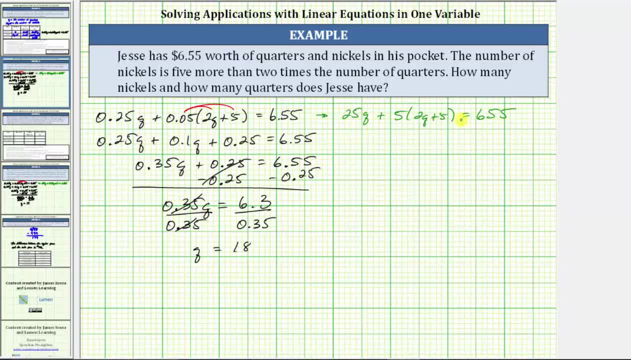 let's take the time and solve this equivalent equation. where the units would have been cents rather than dollars, The steps would be the same. We clear the parentheses here by distributing: This gives us 25Q plus 10Q plus 25 equals 655.. 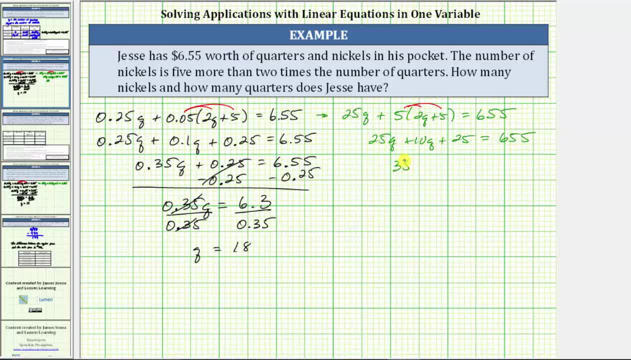 Combining like terms: 25Q plus 10Q is 35Q. Next step: isolate 35Q by subtracting 25.. Again, it's the same step that we took in this equation here, except this equation does not contain decimals. 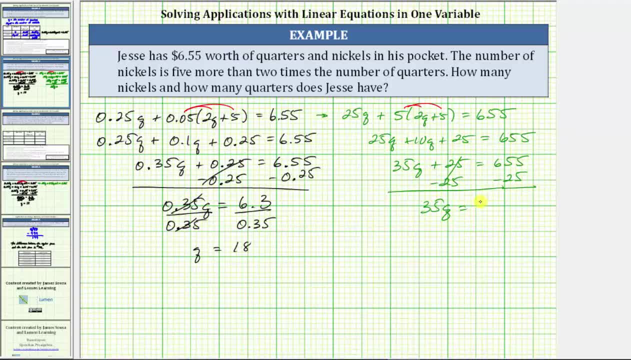 Simplifying, this is zero. we have 35q equals 655, minus 25 is 630, dividing both sides by 35.. Simplifying, we do get q equals 18.. So again we now know the number of quarters is 18.. 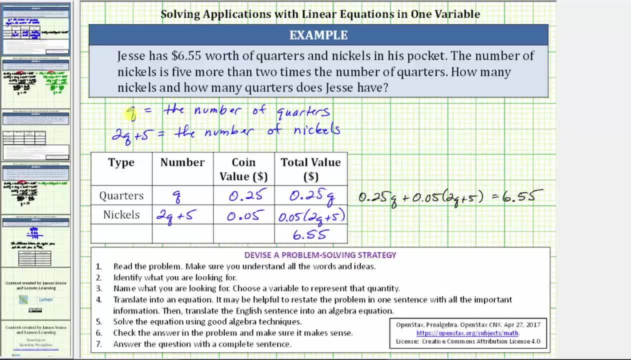 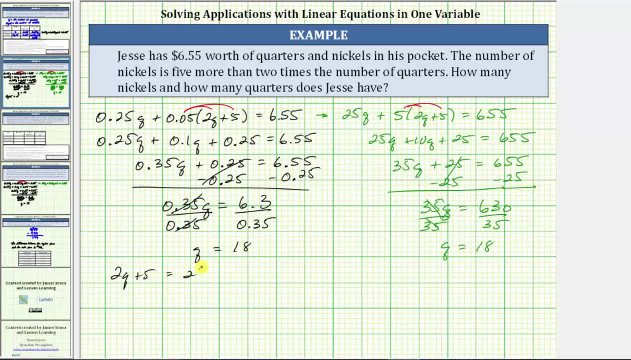 Remember, the number of nickels is two q plus five. so let's determine the number of nickels by substituting 18 for q. Two times 18 is 36,. 36 plus five is 41. So now we know there are 18 quarters and 31 nickels.